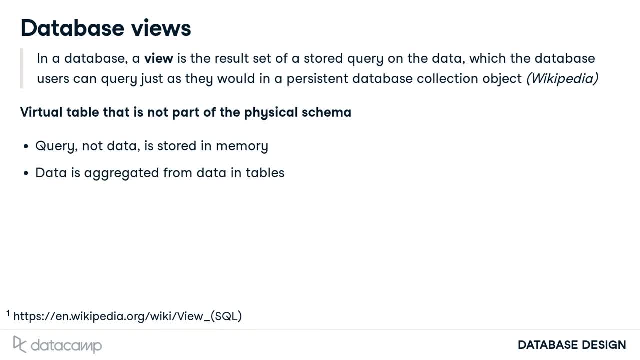 The data in a view comes from data in tables of the same database. Once a view is created, you can query it like a regular table. The benefit of a view is that you don't need to retype common queries. It allows you to add virtual tables without altering the database's schema. 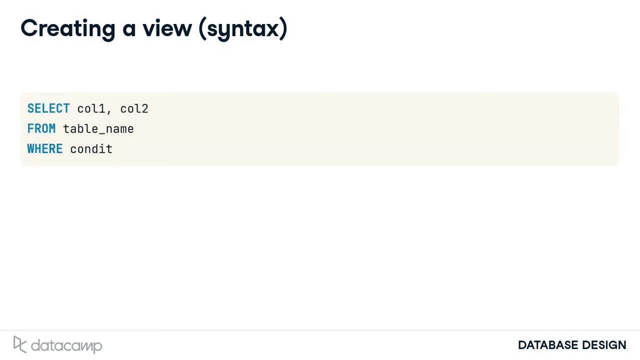 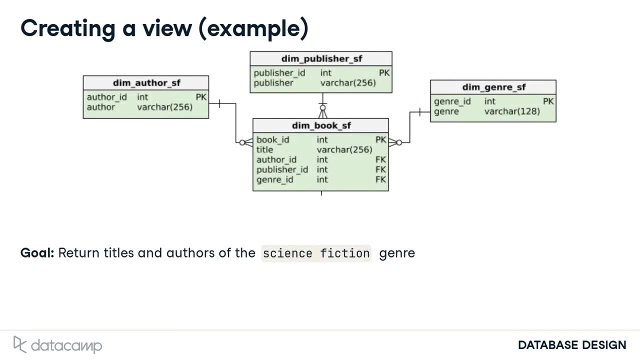 Views are simple to create. You take the query of interest and add a line before it to name the view As such. Here's an example. This is part of last chapter's snowflake schema. Let's say, analysts at your company are often running analytics on the science fiction genre. 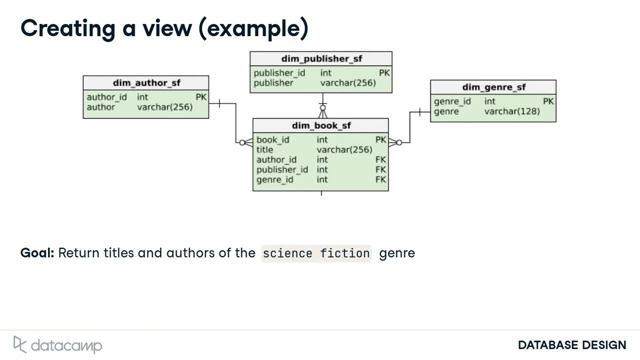 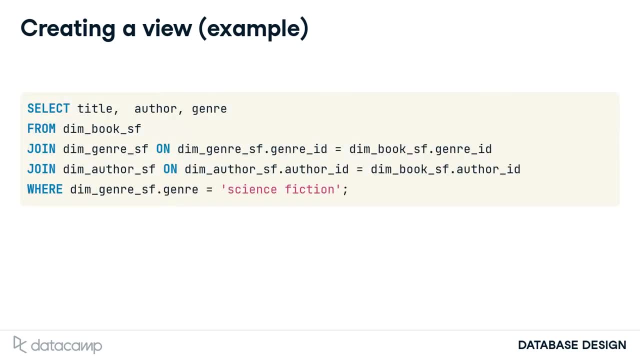 To help their workflow. you want to create a view specifically dedicated to the science fiction genre and its associated book titles and authors. The query would look something like this: To convert this query into a view, you would add a create view statement like so: 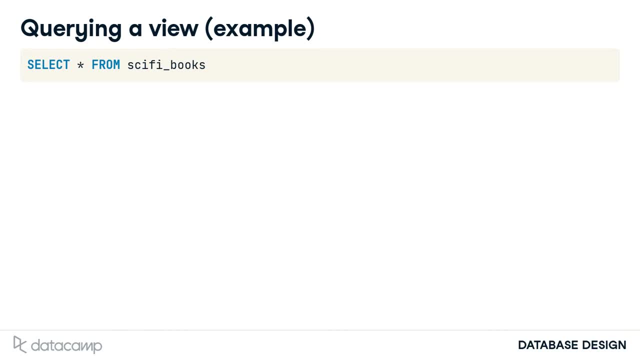 After executing the code from the last slide, you can query the view. Sci-fi books isn't a real table with physical memory. When we run this select statement, the following query is actually being run. It's important to keep track of the views in your database. 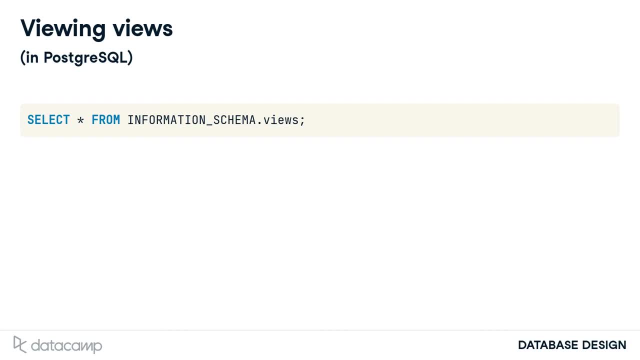 To get all the views in your database. you can run a query on the information schema- dot views table. Note that this command is specific to PostgreSQL. If you're using another DBMS, look at its documentation to find the equivalent command. If you run this command, you will get a long list of views. 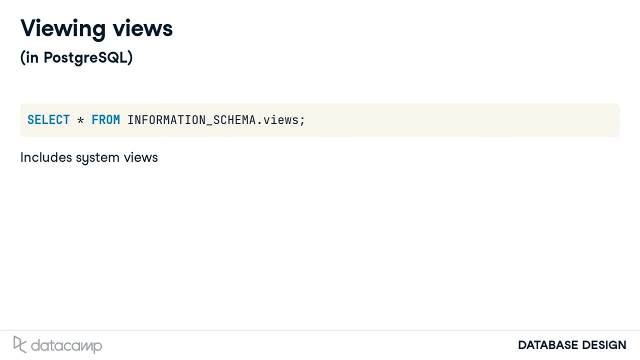 That's because DBMSs have their own built-in views. To exclude system views and to get views that you've created, use this query. It excludes views from PG catalog and information schema, which are built-in view categories. Can you see why views are useful? 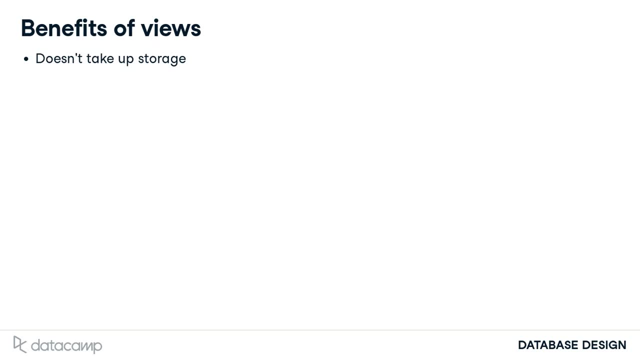 First off, a view doesn't take up any storage except for the query statement, which is minimal. Views act as a form of access control. For example, instead of giving a user access to columns that may have sensitive information, you can restrict what they see via a view. 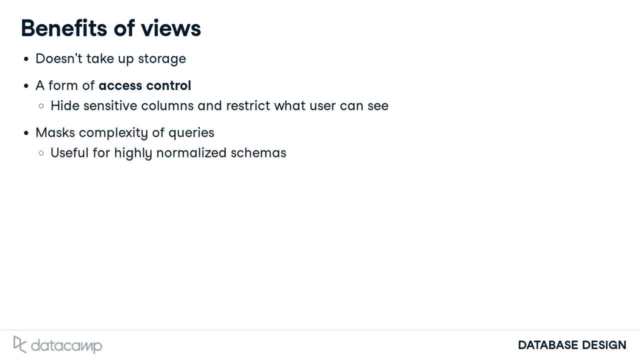 Perhaps most importantly, views mask the complexity of queries. Remember those snowflake schemas from the last chapter and their joins. Views are handy for views normalized past 2NF. You can make those common joins such as aggregating dates or genres into views.